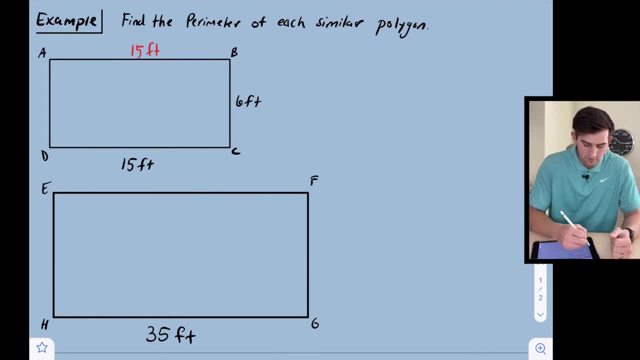 and the width. So we know for a rectangle that would be 15 and this would be six. So we can add these up. We can say 15 plus 15 plus 6 plus 6 and that gives us 42.. So we know our perimeter is 42 feet, for. 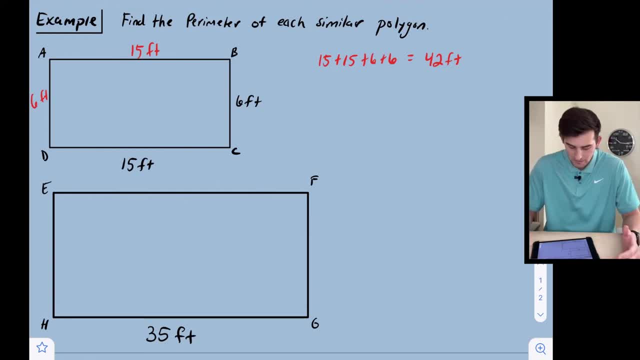 rectangle ABCD. so that's part of our question. But now we want to find the perimeter of our larger rectangle or our similar rectangle, So we can take a side, two side lengths that we know, 15 and 35, and we also know the perimeter of the. 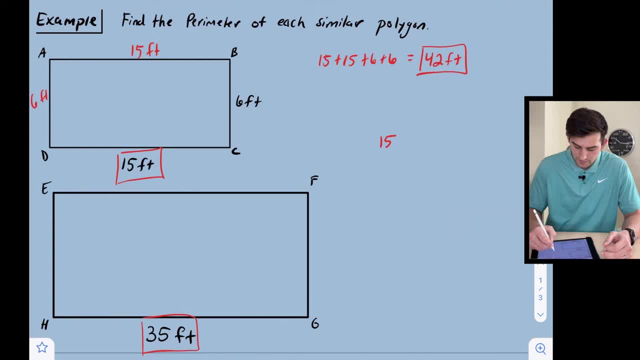 first shape. So we can say 15 over 35 is equal to 42 over X, because X would represent the perimeter of our larger rectangle here. So we can cross, multiply and we can do 15 X equals, and we can do 42 times 35 and we get 1470. and then we 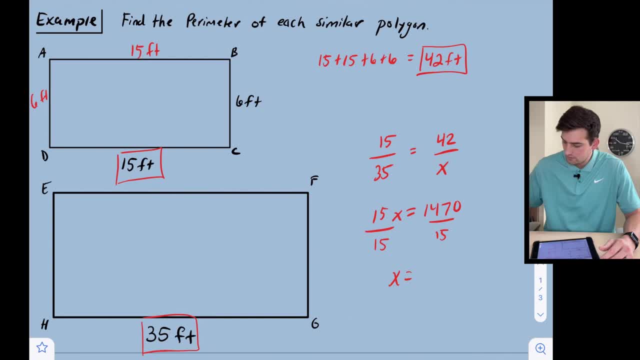 can divide by 15.. So we get X equals divided by 15 and we get 98.. So we get 98 over 35, and then we can divide by 15.. So we get 98 over 35, and then we get for the perimeter of the larger shape, and so now we have the perimeter of the. 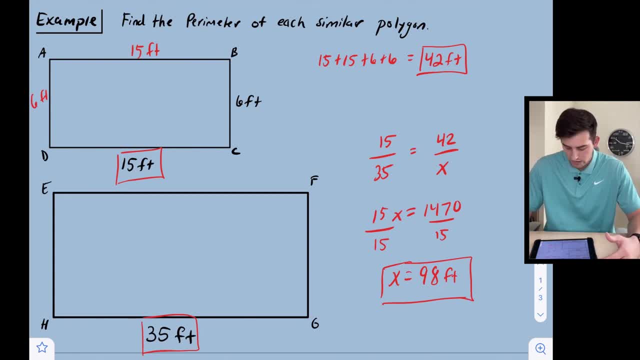 small shape, 42 feet, and we have the perimeter of the large shape, which is 98 feet. Okay, so that's how the perimeters of similar polygons are related.